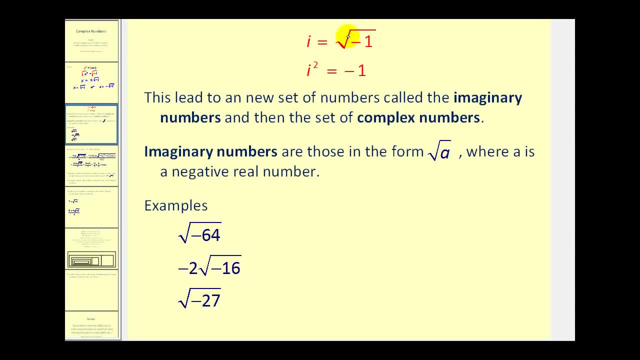 very similar to how we simplify square roots, except now we have a new definition to deal with the negative, So we could rewrite this as the square root of negative 1 times 64, which is equal to the square root of negative 1 times the square root of 64.. Well, now by 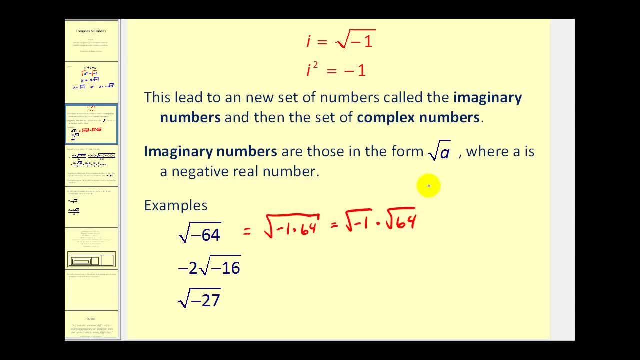 definition. this is equal to i, This is equal to 8, so this simplifies to the imaginary number 8i. On this next one, this is negative 2 times the square root of negative 16.. It's negative 2 times the square root of negative 1 times 16.. So really it's very. 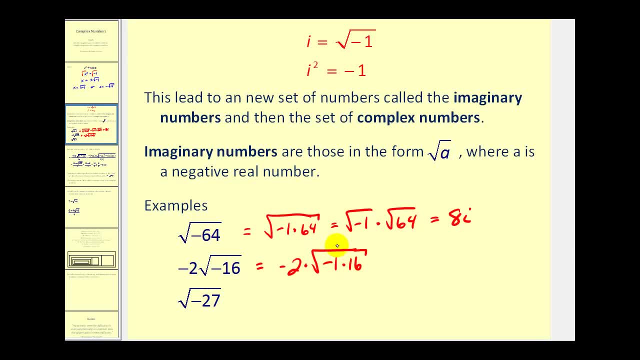 similar to what we've been doing in the past with square roots. We just have an extra factor of negative 1 which gives us an i. So you can probably see this would be negative 2 times. this would be equal to i. this would be equal to 4.. So we'd 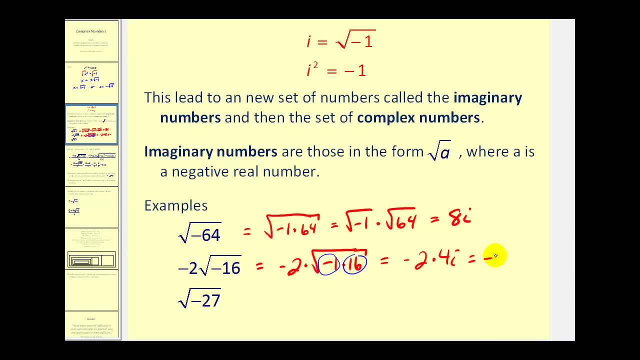 have negative 2 times 4i, which is equal to negative 8i. The square root of negative 27 is equal to negative 1 times 27.. 27 is not a perfect square, so it would be 3 times 3 times 3.. So the square root of negative 1 simplifies to i. The square root of 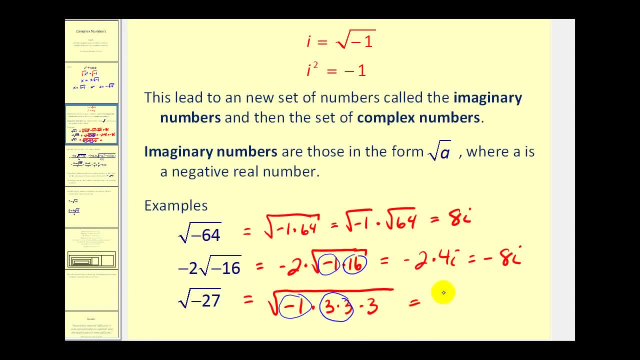 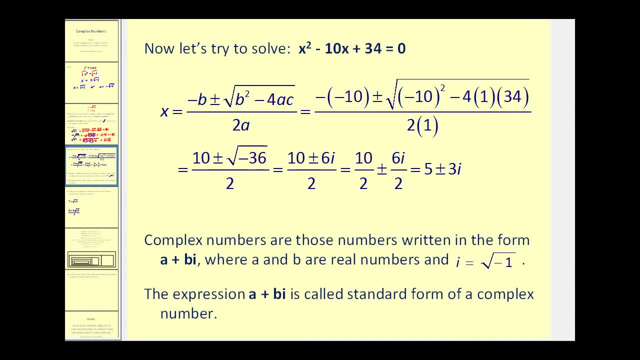 9 simplifies to 3.. So this would give us a 3i, and then we're left with square root 3.. Now if we try to solve the equation, x squared minus 10x plus 34 equals 0. That also doesn't factor, so we would apply the quadratic formula. I've already 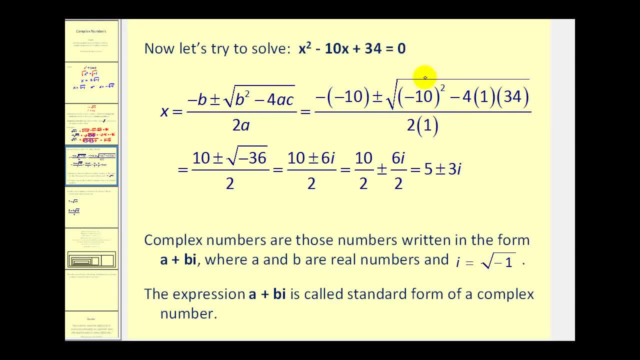 done this to save some time. but what's new about this is, when we simplify the discriminant, we end up getting the square root of negative 36, which leads to part of this answer being imaginary. So we have 10 plus or minus 6i all. 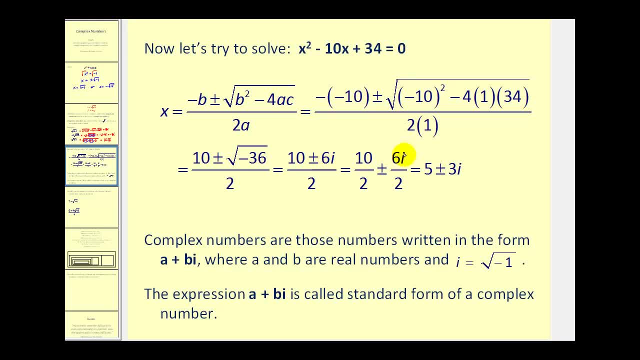 divided by 2.. We divide both terms and numerator by 2. We have 5 plus 3i. So there is an imaginary number as part of this solution, but there's also a real part, and that led to another set of numbers called the complex numbers. Complex numbers are those numbers written in the 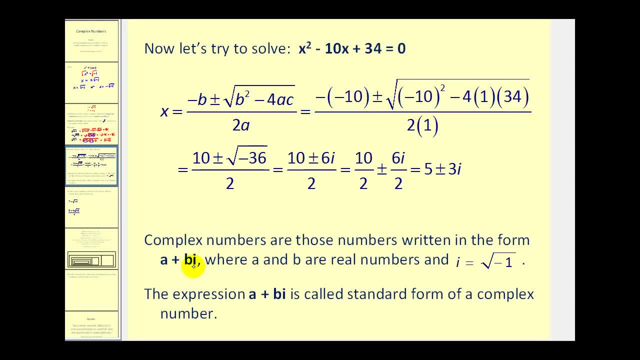 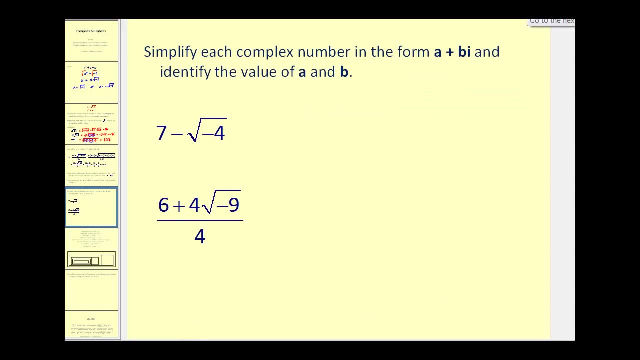 form of a plus bi, where a and b are real numbers and i is the square root of negative 1. So we have a real part, that's the a part, and we have the imaginary part, the bi part, and a plus bi is called the standard form of a complex number. So if 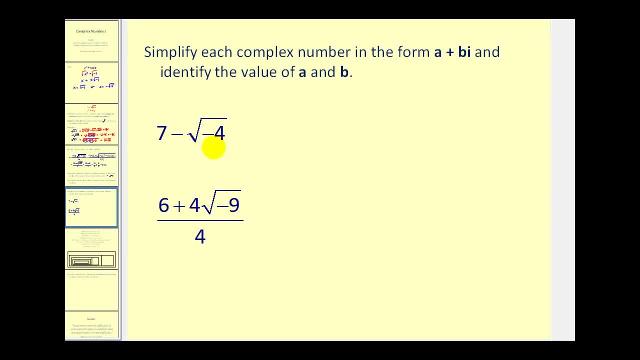 we wanted to simplify these complex numbers in the form of a plus bi. we still need to simplify the imaginary part. So we'd have 7 minus square root of negative 1 times 4.. We know now this will give us i. We know the square root of 4 is 2.. So this would 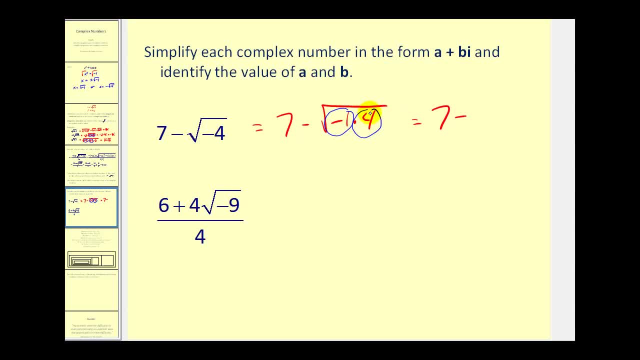 simplify to 7 minus 2i, And again it's in the form of a plus bi. Let's take a look at one more here. After you do these a while, you probably look at that and see 3i, but for the purpose of showing work, let's go ahead and rewrite. 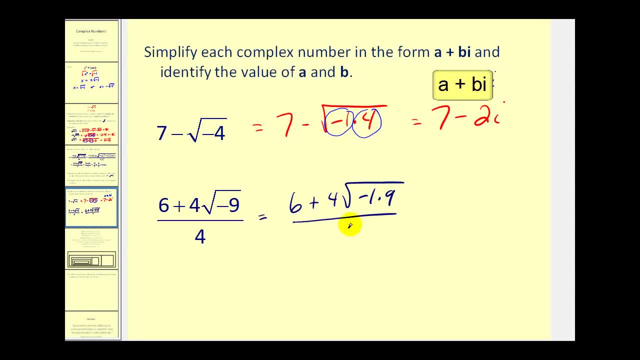 this as negative 1 times 9 all over 4.. So we'd have 6 plus now the square root of negative 1 will give us i. The square root of 9 will give us 3.. This is equal to 3i. 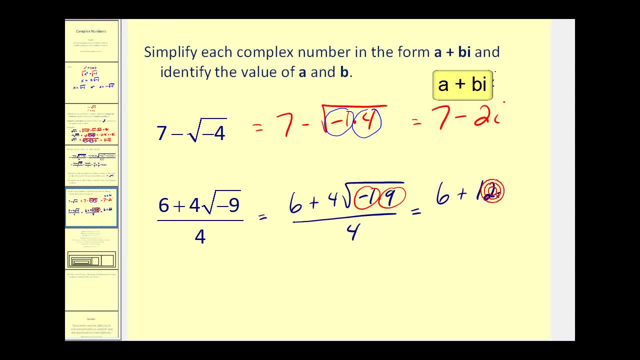 times 4.. That would be 12i, 12i, 12i, 12i, 12i, 12i, 12i divided by four. Now be careful simplifying here. We cannot just simplify the six and the four. 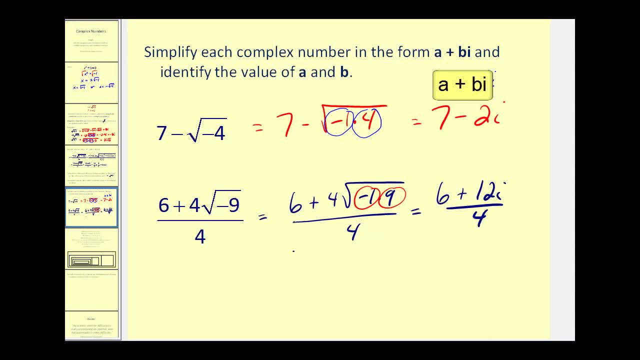 We cannot simplify across addition, So we should rewrite this as two separate fractions: Six divided by four, plus 12i divided by four. This gives us three halves plus three i, Again in the form of a plus bi. Let's take a look at how the sets of numbers 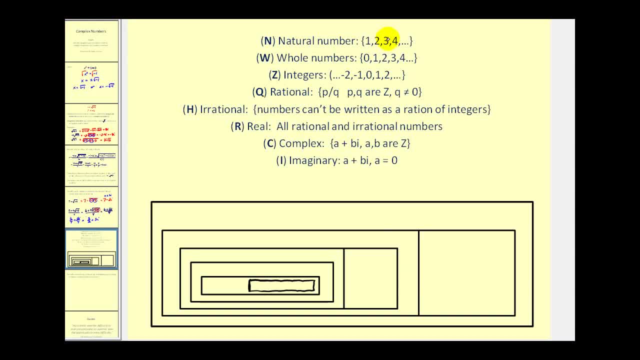 relate to one another with a Venn diagram. Here we have the natural numbers, whole numbers, integers, rational, irrational numbers, real numbers and the new sets, the complex numbers and the imaginary numbers. And now that we know that complex numbers, 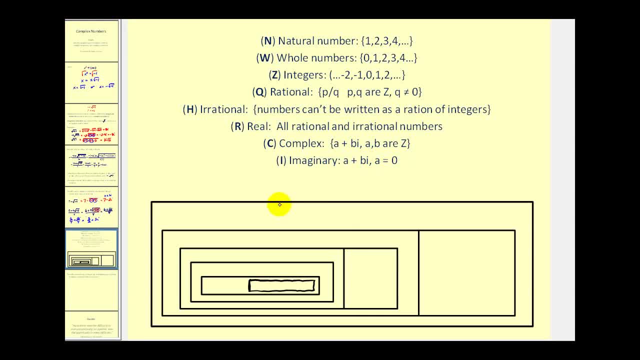 have both a real part and an imaginary part. you can see that this is going to be the most encompassing set of numbers, So the complex numbers would be out here in the form of a plus bi. Next, since the complex numbers are made up of a real part and an imaginary part,